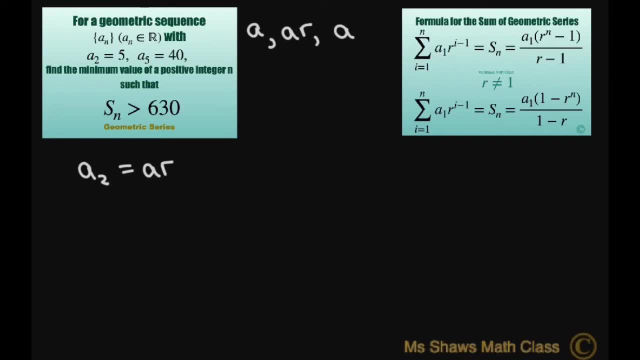 The third term would be a times your common ratio two times, so that would be squared, So that equals 5.. And our fifth term is going to be similarly your first term. times common ratio four times, So r to the power of 4, and that equals 40. Now, this is equation 1 and equation 2.. 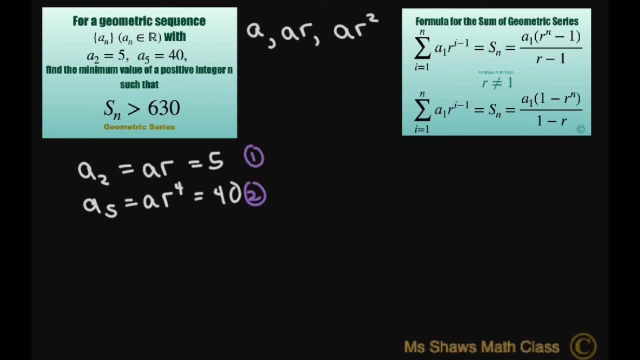 So what we want to do is solve for r and a, so we can use this formula here. All right, so let's divide 2, divide it by 1.. All right, so we take a r to the power of 4 equals 40, divide it by the second term, so that's going to be a r and 5.. 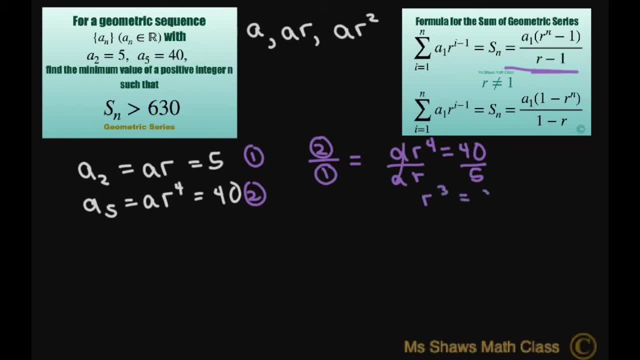 So the a's cancel and you get r cubed equals 8,. therefore r equals 2.. All right, so since r is 2, to find a, let's just substitute it in here. We need our first term. So a times 2 equals 5, so our first term is 5 divided by 2.. 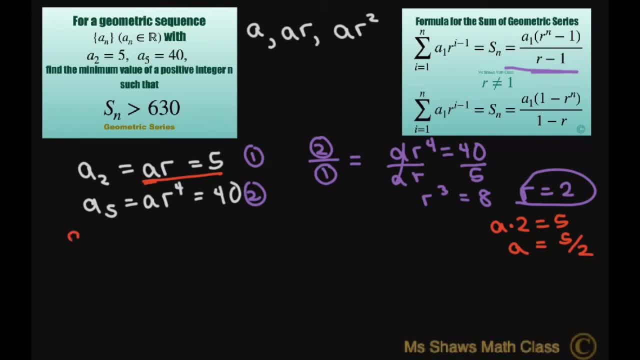 All right. so since we have that, we can use our sum- It's going to be our first term here- which is 5 halves, and then our r is 2 to the power of n minus 1, all divided by 2 minus 1.. 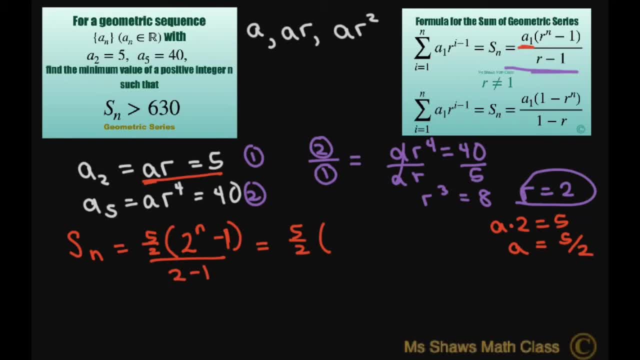 All right, so we're going to use our first term here, which is 5 halves, and then our r is 2 to the power of n minus 1,, all divided by 2 minus 1.. So this equals 5 halves times 2 to the power of n minus 1, and this has to be greater than 630.. 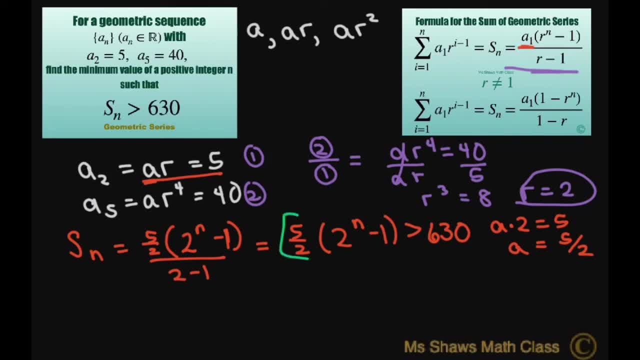 All right. so let's multiply both sides through by 2 fifths and that's going to give me 2n minus 1 has to be greater than 252.. when you multiply those so you get 252, or when you add 1 to both sides.